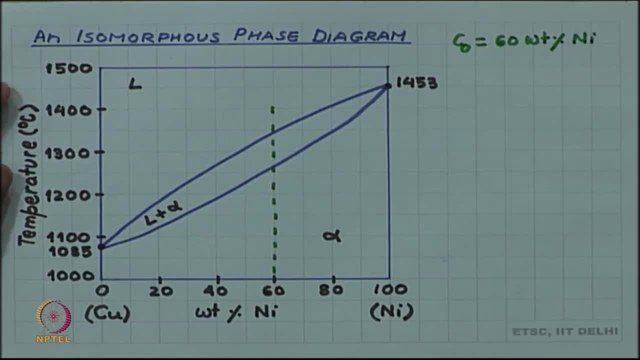 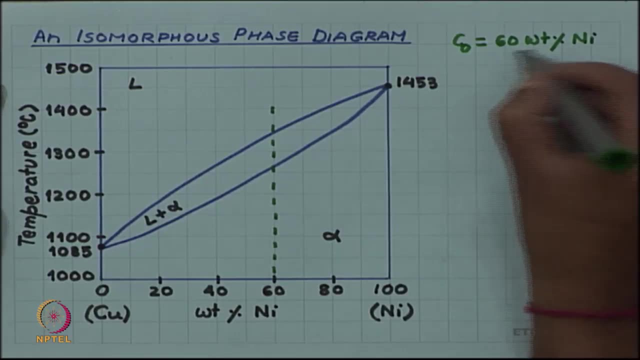 percent nickel. remember that we are having binary alloy, So only one component need to be specified: 60 weight percent nickel automatically tells us that the remaining 40 weight percent is copper, Because we are talking of copper nickel system. So either 40 weight percent copper or 60 weight. 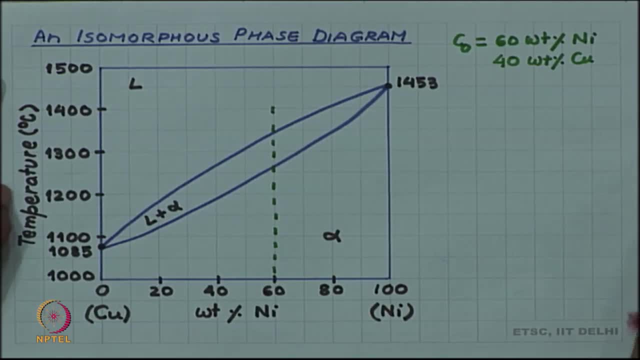 percent nickel can be used as composition. we have labeled the composition axis as weight percent nickel, So we will use 60 weight percent nickel. So that is the composition of the alloy. if this alloy is at a high temperature- and by high temperature we mean above the 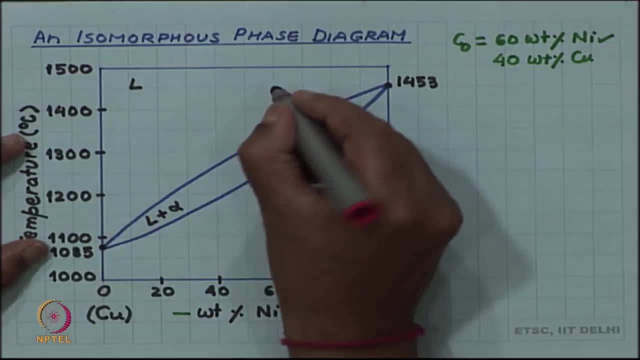 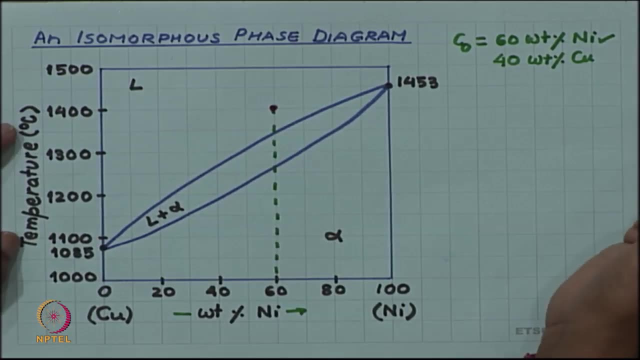 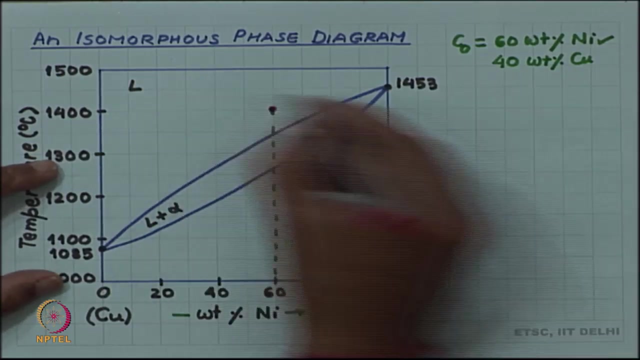 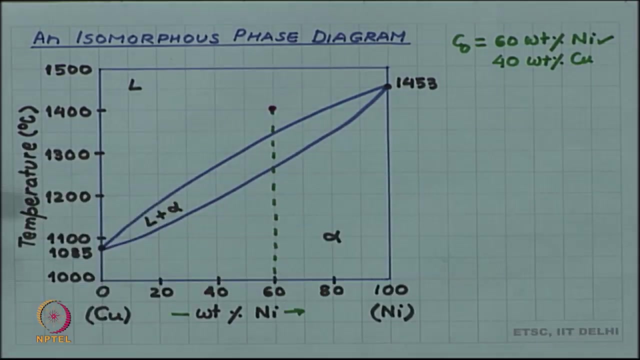 liquidus temperature. So suppose it is at this temperature, then the phase diagram tells us that the phase present is the liquid phase. So the entire phase here will be a liquid phase. So if I draw the diagrams in terms of what you will see in a, what you will see in a sample, let 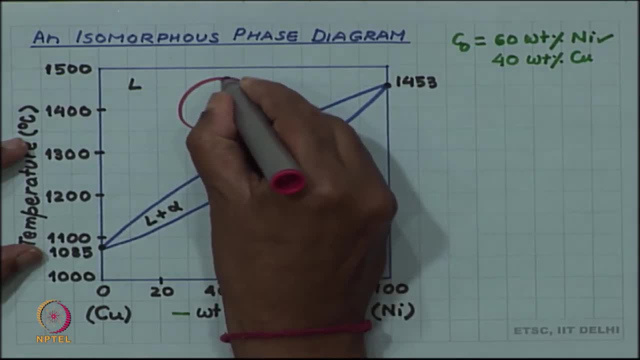 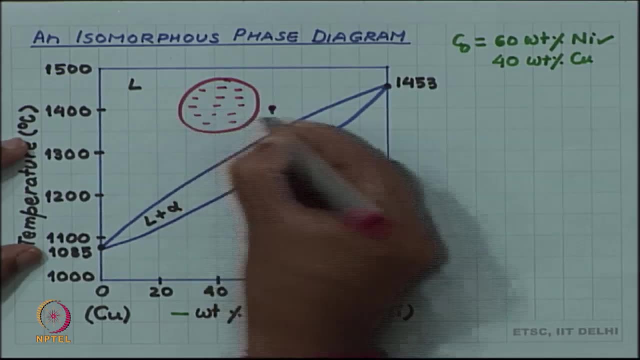 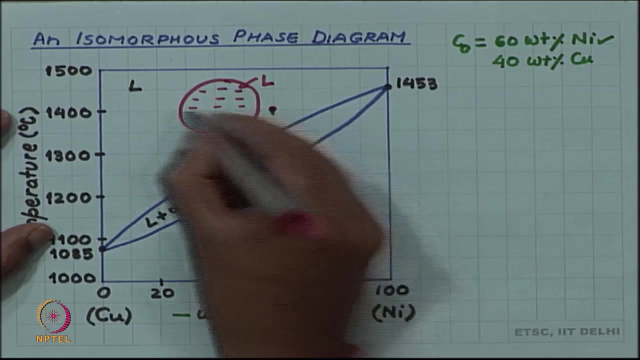 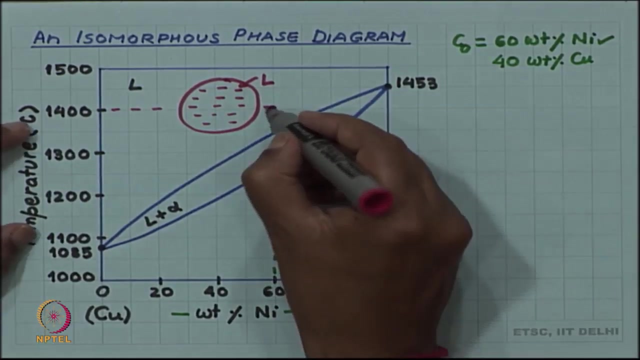 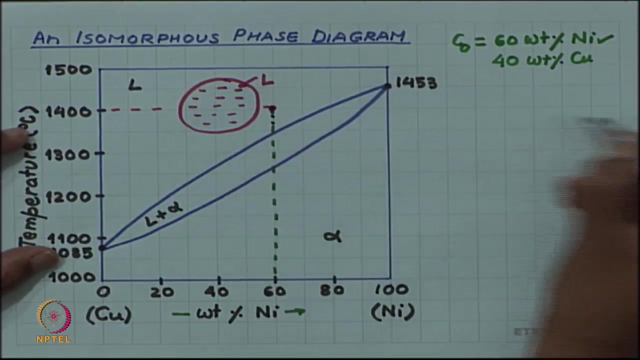 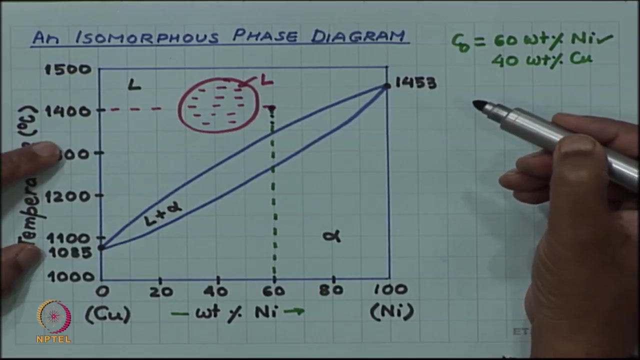 me draw it. So all you will see is the liquid. So the entire alloy is the liquid phase at this temperature, 1, 4 t, 100 degrees Celsius. as you cool, the alloy will. For example, there will be thermal contraction, so the volume of the liquid will reduce liquids. 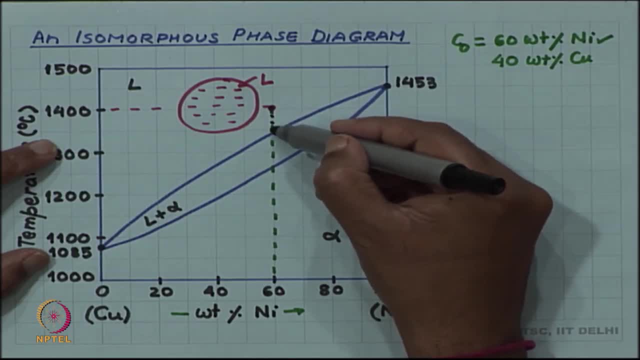 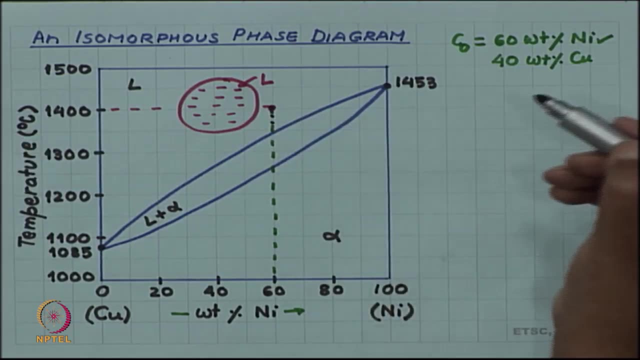 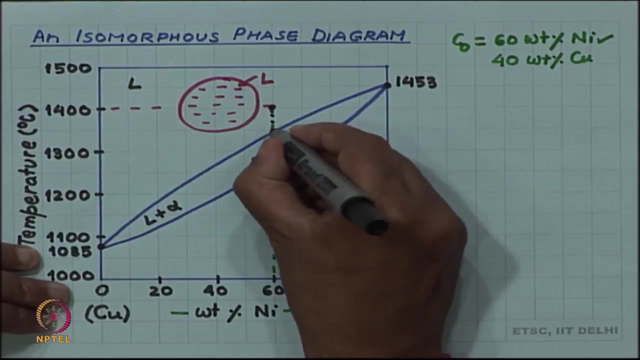 generally will increase in viscosity as the temperature lowers, so the viscosity will increase. So such physical properties will change, but there will be no phase change till you reach the liquidus boundary. So the liquidus boundary is reached at this temperature and we can call that temperature. 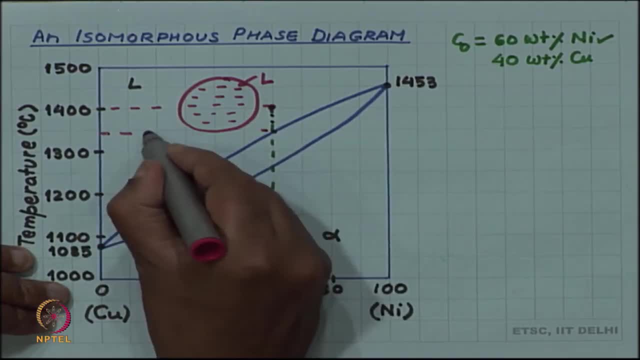 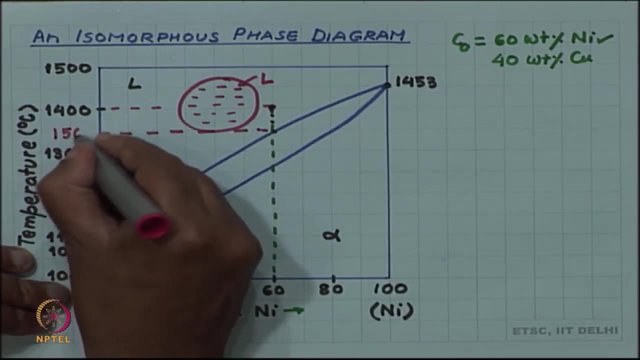 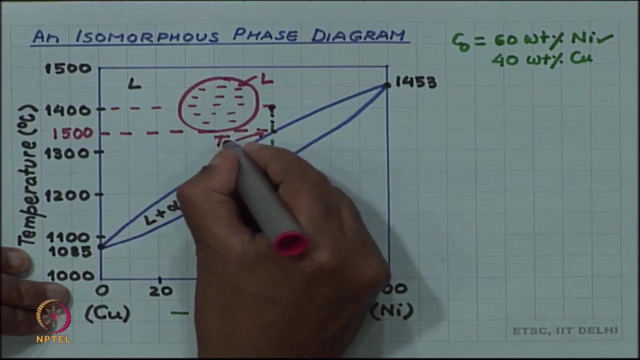 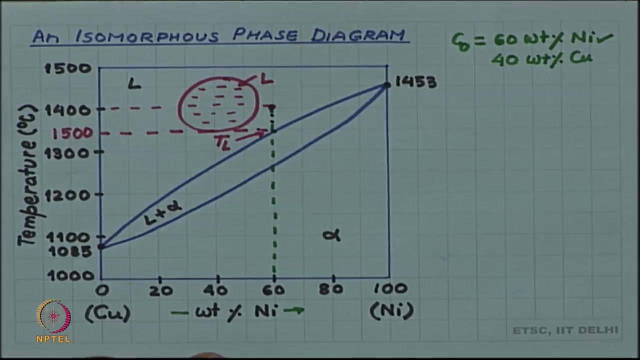 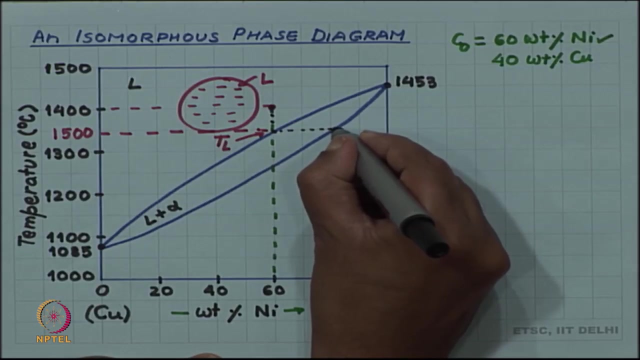 as the liquidus temperature. So in this diagram is approximately 1500, so 1500 is the liquidus temperature. let me label it as T L. So when the alloy, So when the alloy reaches the liquidus temperature, you will start having, start begin to see a 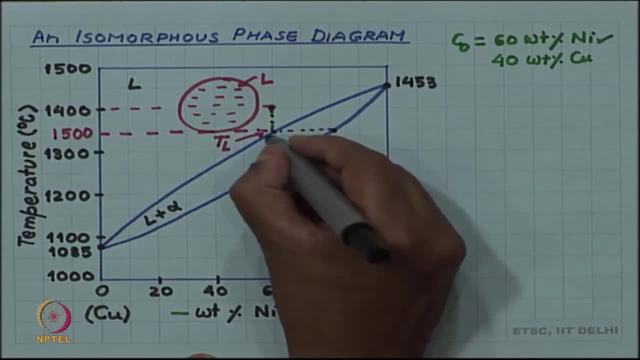 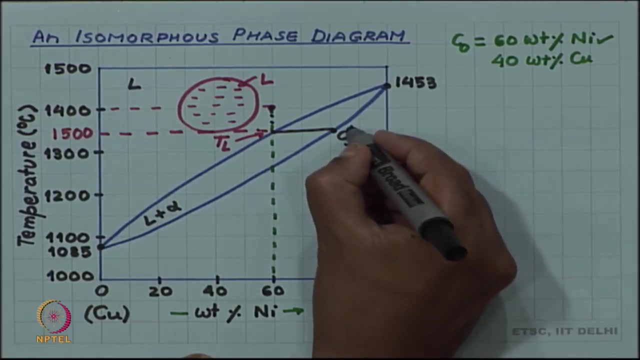 first solid and by tie line rule, the first solid will have a composition given by this point. Let me label. I have drawn a horizontal, which is the horizontal tie line. you have learnt in the previous class, So let me call that CS. Let me table it as one. 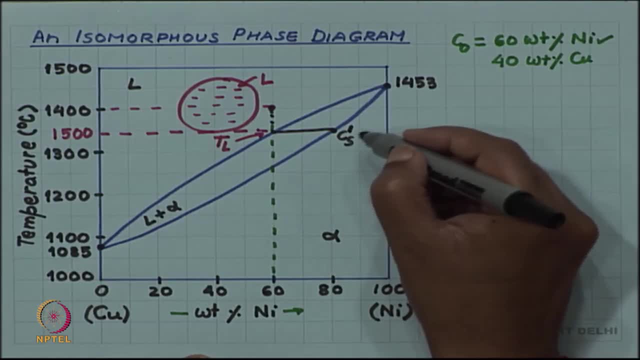 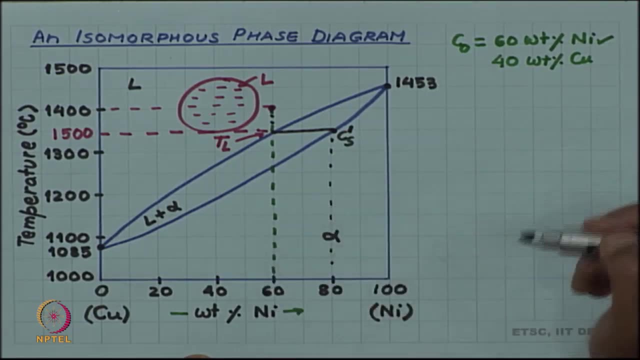 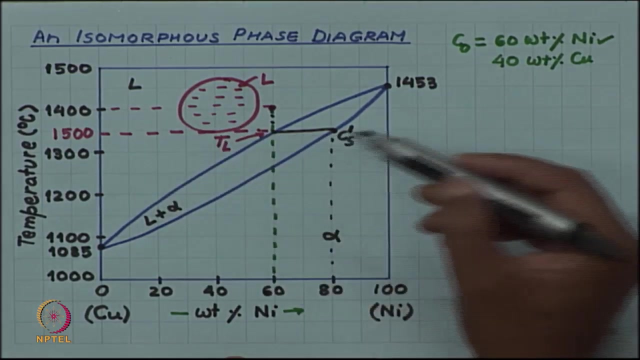 That is the first composition solid which will form. in this diagram you can read- I am not intending to tell you that this is exactly the- because I have drawn this phase diagram by hand. So these compositions I am using as example and these temperatures I am using an example. 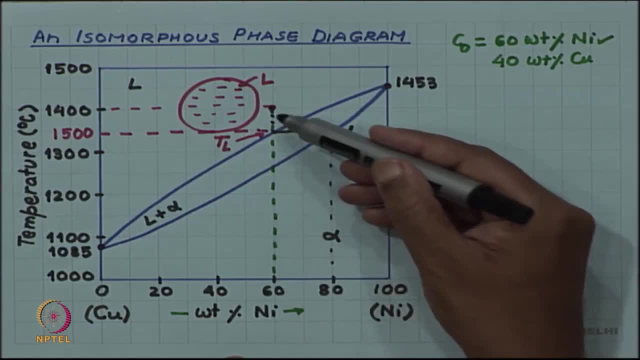 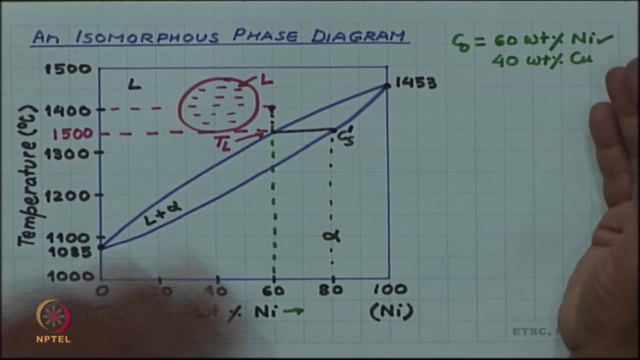 it is not that in the actual phase diagram for 68 percent Тоist weight percent alloy, 1500 degree Celsius is the exact liquidus temperature. So you have to see the real published phase diagram which is available in text books and manuals and nowadays on internet also. 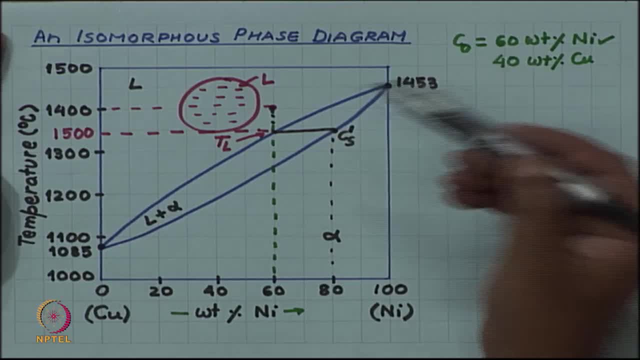 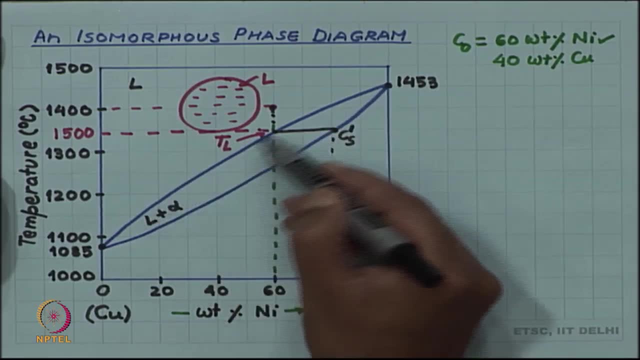 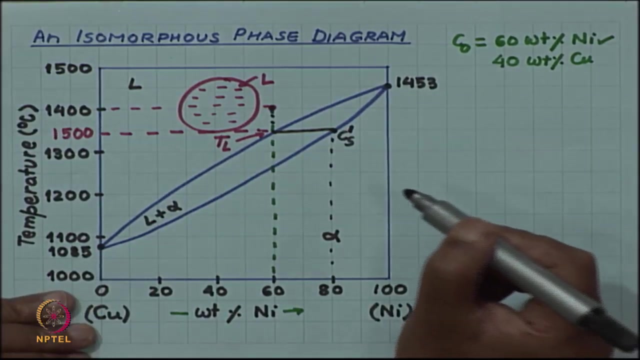 So you can look that up here. I am taking it as an example that if this vertical line, the alloy composition vertical, intersects the liquidus boundary at whatever temperature that is the liquidus temperature And for example, say: I have taken this to be 1500. similarly, wherever this horizontal, 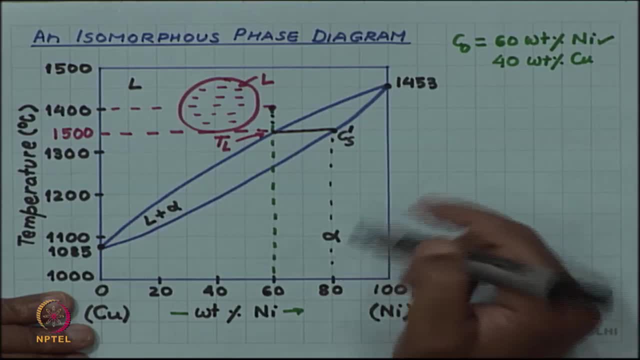 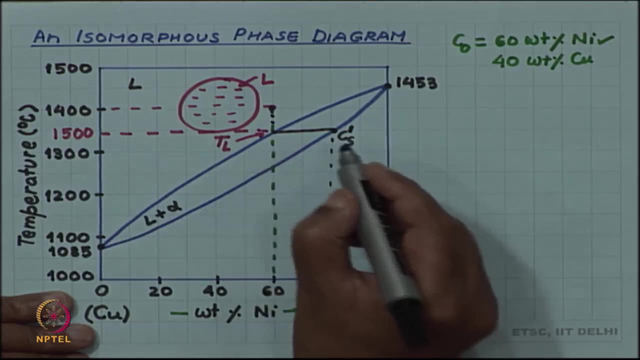 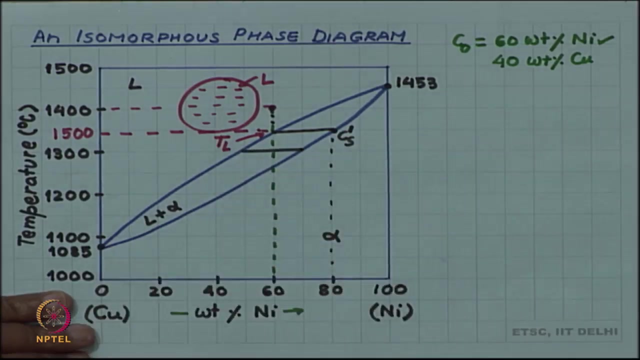 cuts the solidus line, that is the first solid to form, and again, for example, say: I am taking it to be the 80 percent. Then, as you now lower the temperature, as you now lower the temperature, you have seen that the fraction of the solid is given by the opposite lever arm. 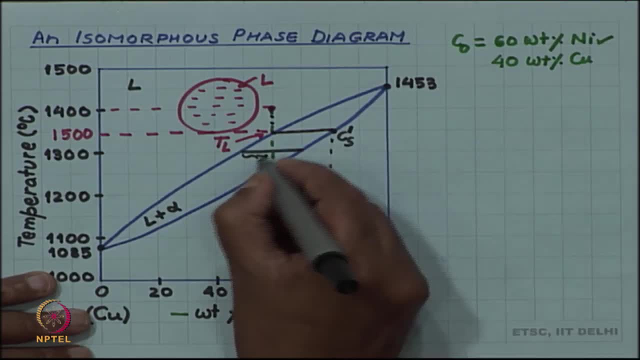 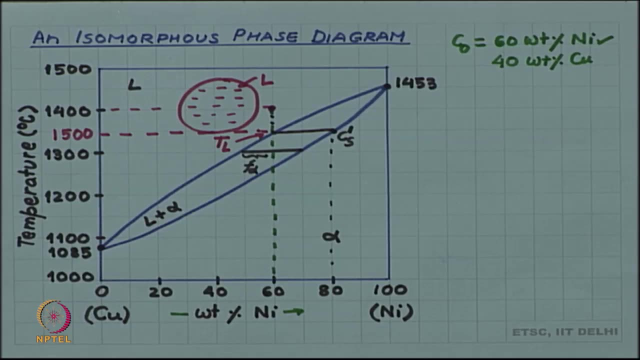 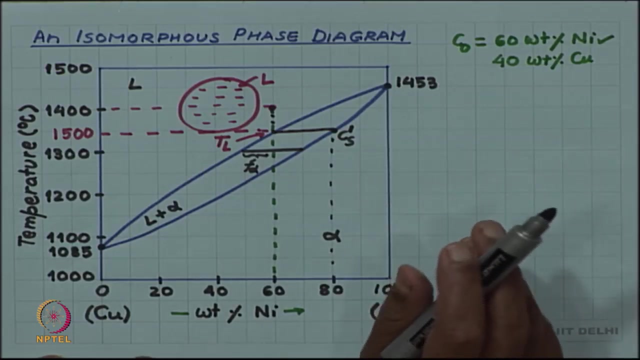 So since solid is on my right side, alpha is on right side, the left side lever arm will be proportional to the fraction of the solid phase and by lever rule this arm divided by total arm will be the actual fraction of the solid phase. So you can see here if I really apply the tie line rule. 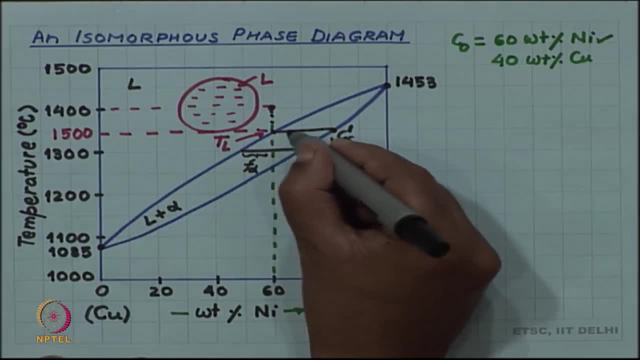 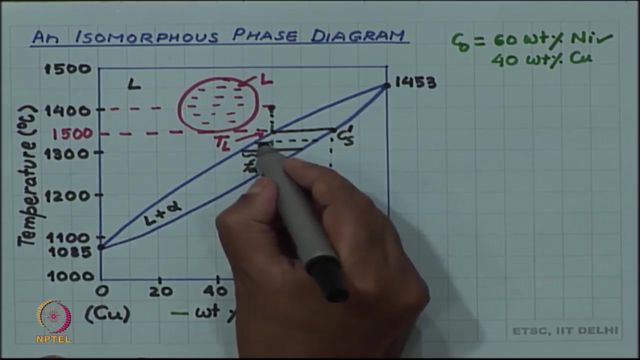 So my f alpha arm was really 0. So the first solid is just going to begin Only if you lower the temperature a little bit, then you have a small arm. if I draw at an intermediate temperature, you can see that the f alpha arm which is in this case is this: 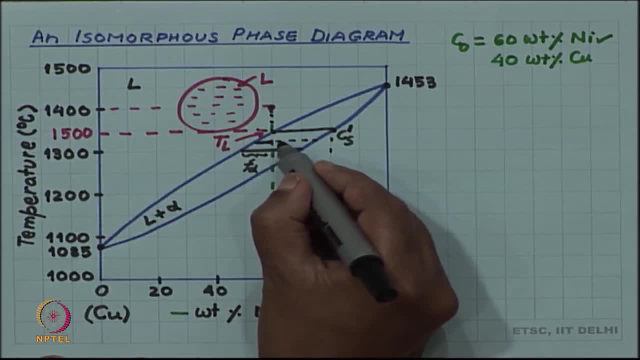 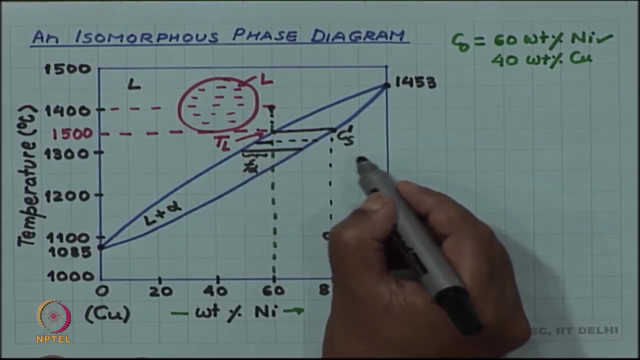 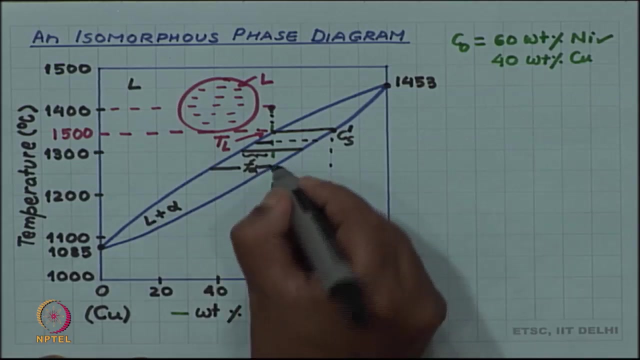 much divide by the total arm is a smaller fraction, and as you lower the temperature you get higher fraction of solid. So this is how the solidification is progressing: that as you lower the temperature you will get more and more solid, And finally, when you reach a temperature corresponding to where the composition vertical. 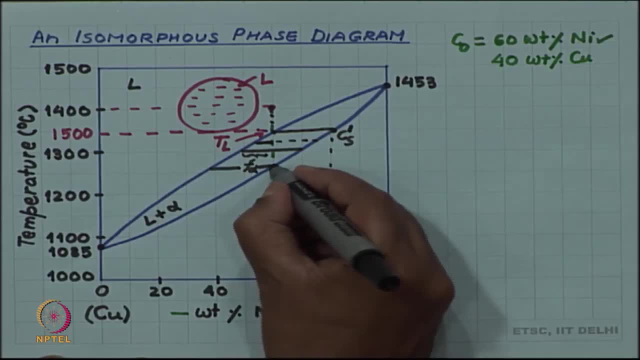 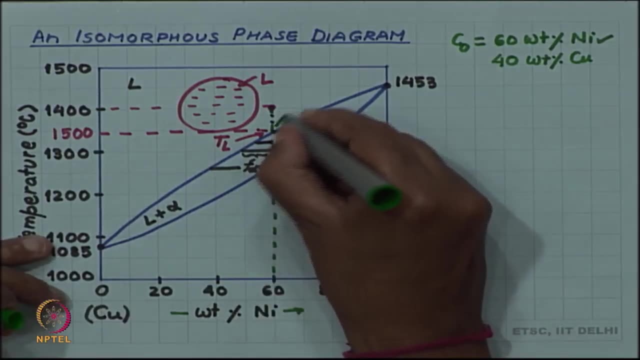 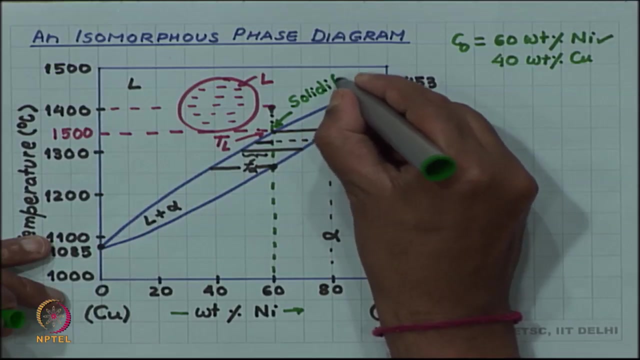 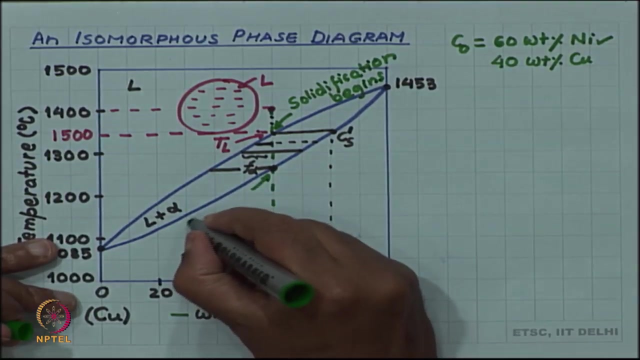 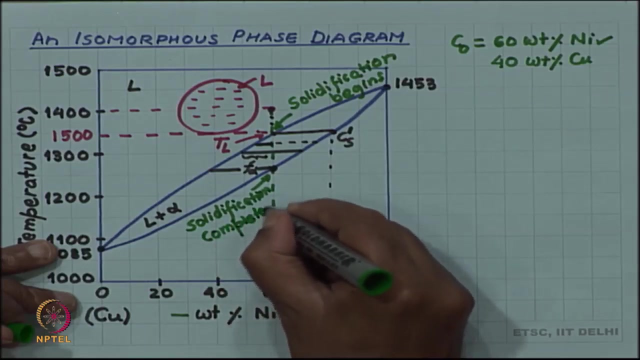 hits the solidus boundary, at that temperature the solidification will complete. So we can write this it where it intersects the liquidus boundary. that is where solidification begins and where it hits the solidus boundary, the solidification completes, solidification completes. 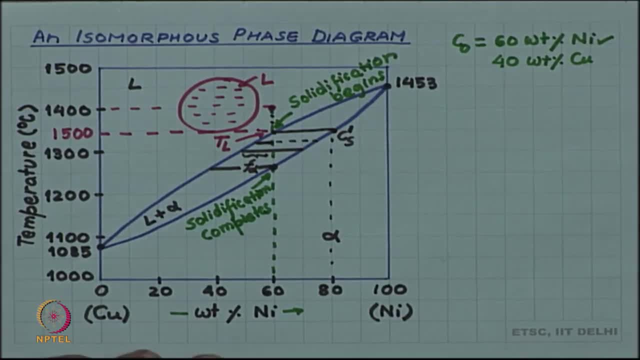 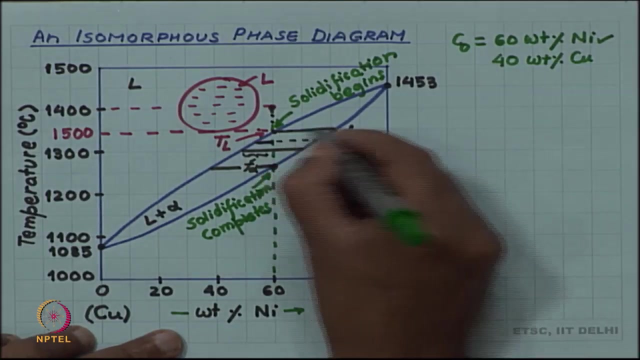 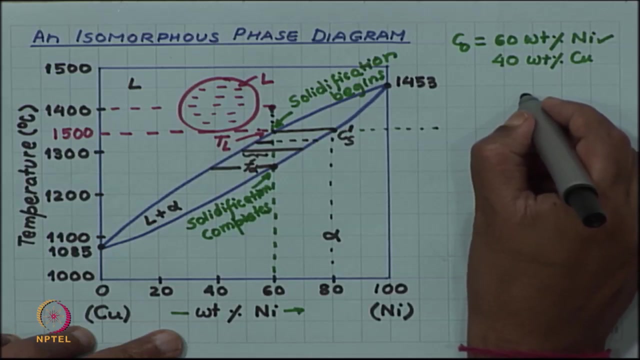 so this is the progress of solidification. that So, if I try to draw a few more diagrams, like I draw for the liquid one, So just at this T L temperature, the diagram will look something, in fact just slightly, below T L. 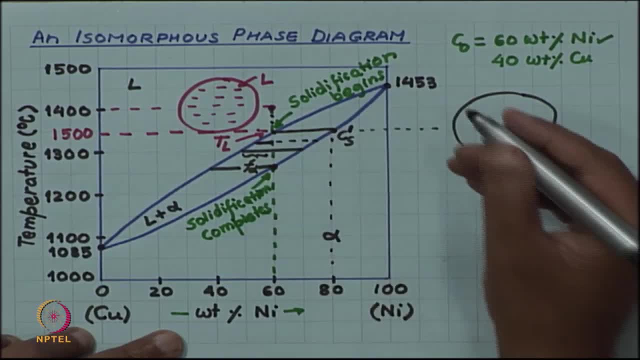 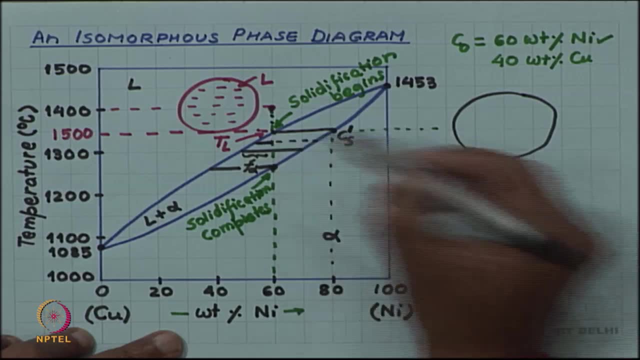 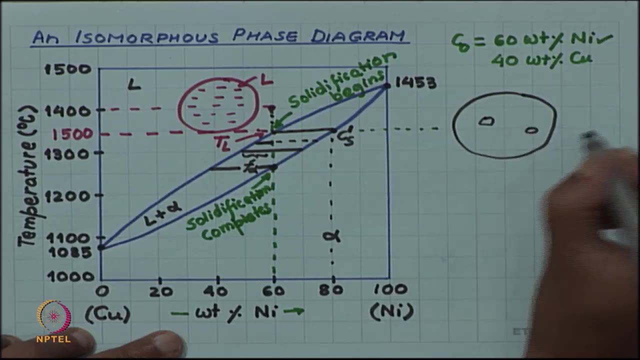 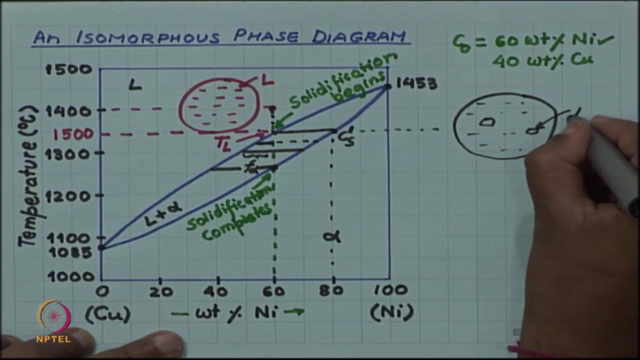 So T L we are taking as a limiting case of beginning of solidification. but since the lever arm F alpha is 0, there actually there is no solid at this point. solid just begins if I lower the temperature. So there will be a small amount, a very small amount of solid just going to begin solid. 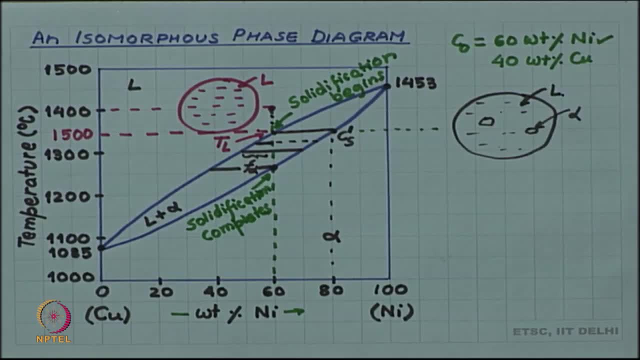 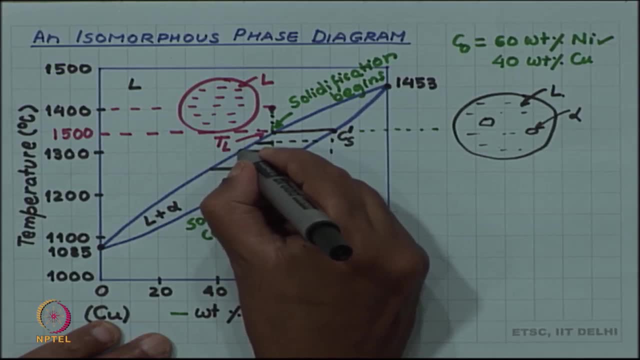 is alpha, Then as we have lowered, you can see the tie line also gives the end point of the tie line gives you the liquid composition and the solid composition. So the liquidus end of the boundary gives you the liquid composition and the solidus. 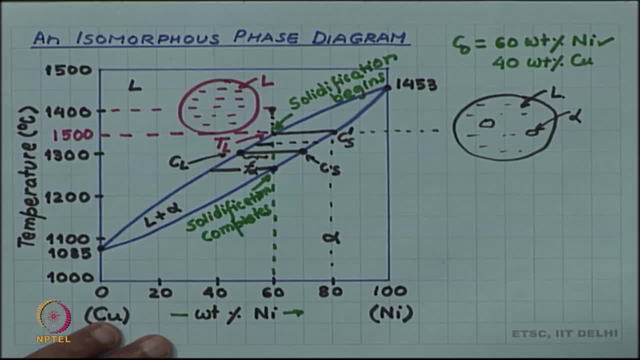 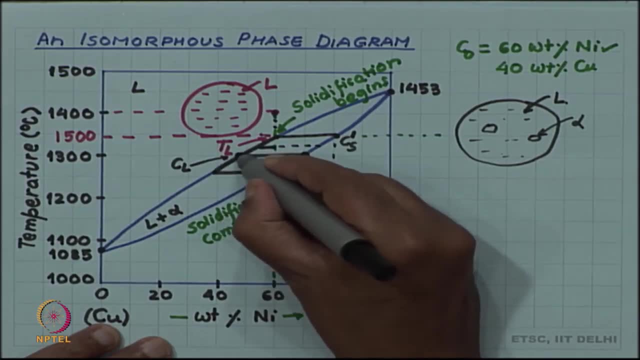 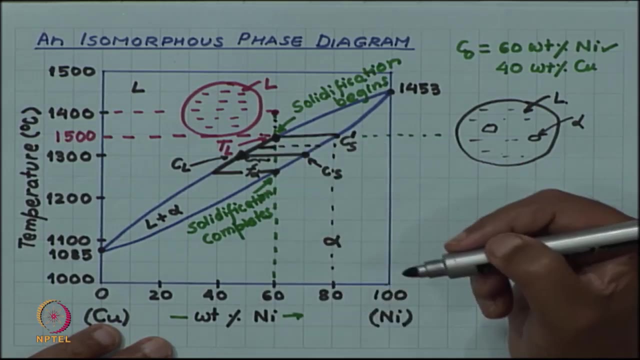 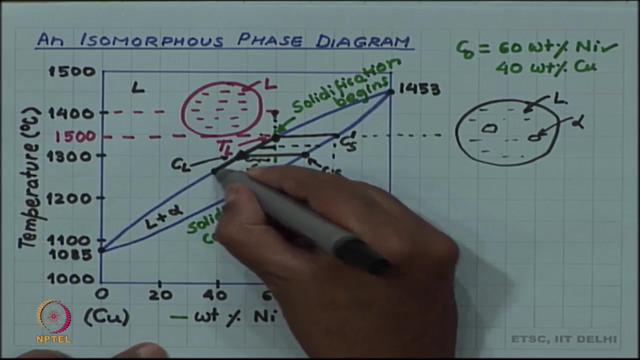 end of the boundary gives you the solid composition. So you can see that both the liquid and solid compositions evolve along these lines. Okay, Okay, So initially the liquid composition was same as the starting liquid, but gradually liquid depletes in nickel and the final liquid, which is solidifying, is of much lower concentration. 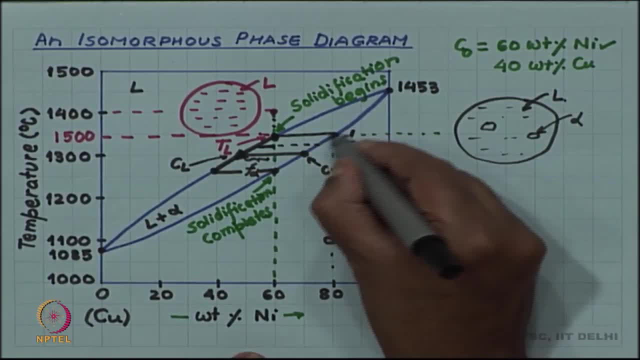 than the original alloy. Same thing happens with the solid also. so the solid composition evolves along the solidus line. So the first solid to form was the solidus line. So the first solid to form was the solidus line. 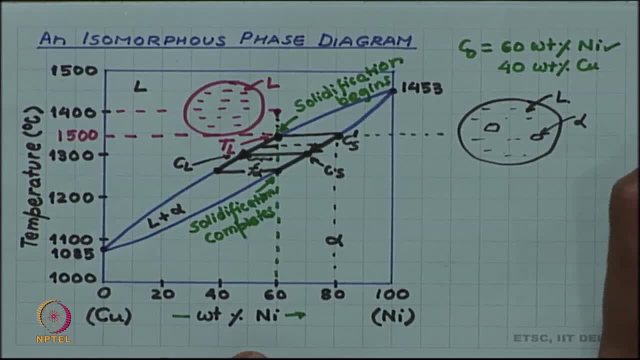 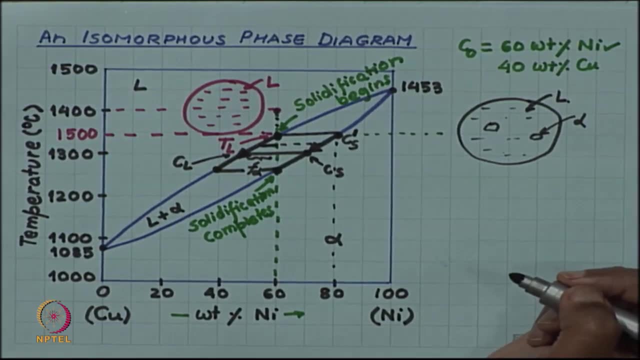 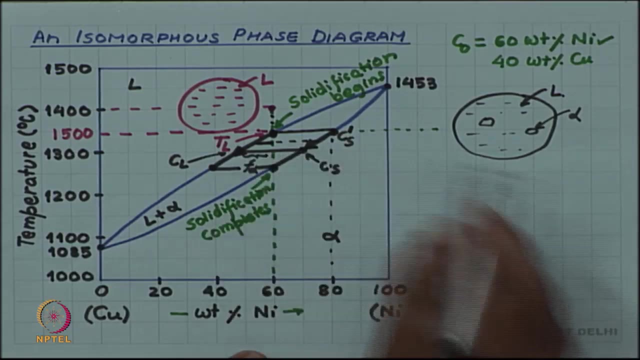 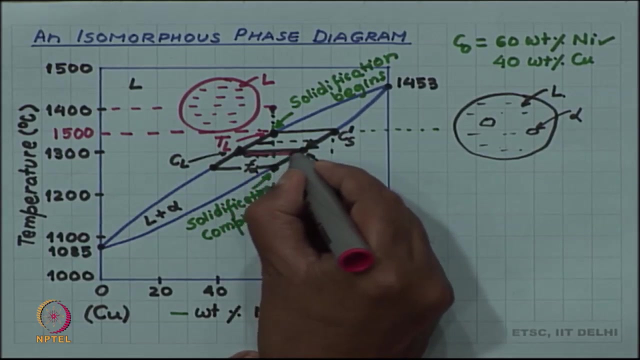 Okay, So this is the C S 1 which I have written. but the final solid which is forming is of composition, same as the alloy composition. So the composition changes as the solidification is happening. and at this temperature, at this intermediate temperature which we are now considering, you can draw the tie line and 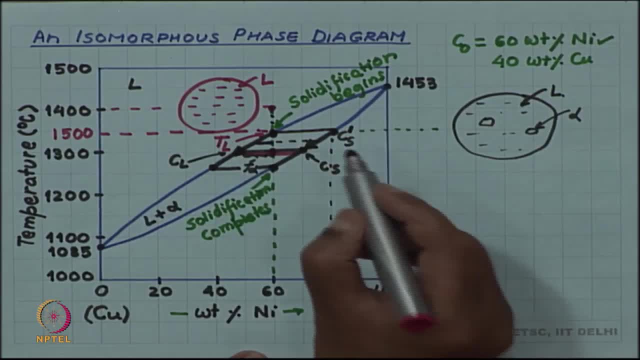 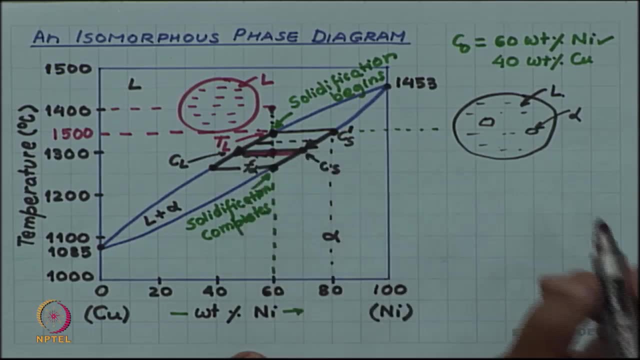 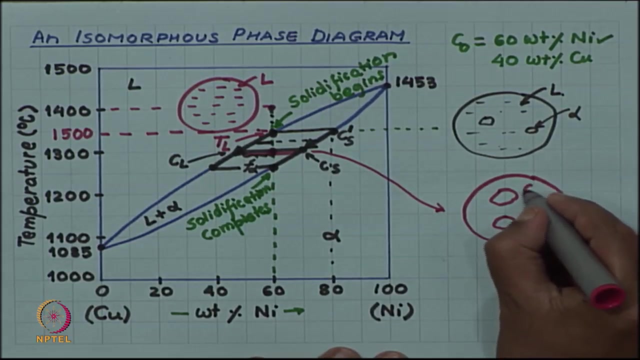 find out what is the fraction of alpha, Okay, and the fraction of liquid. In my drawing it is more or less. you can see that the two lever arms are the same. So I can imagine that at this temperature I have 50 percent solid and I am showing several chunks and not I am not making 50 percent. 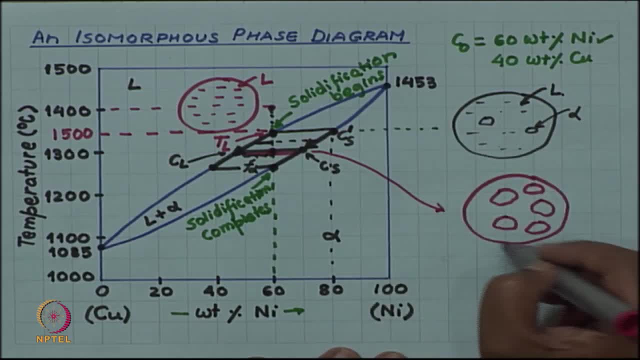 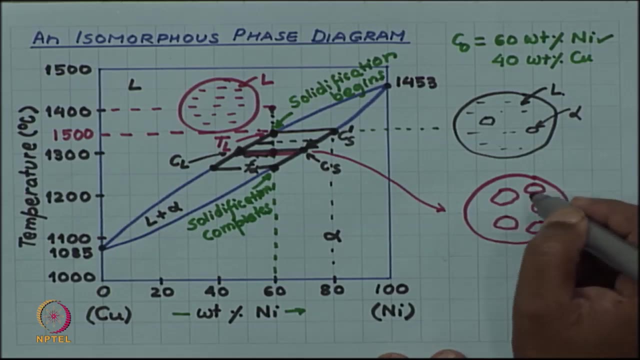 solid as one single half of the diagram as solid and another half as liquid. I am showing several chunks because this is how the physical process develops, that there are several nucleation sites at which solid begins to form. So it is not that only solid will begin at, only 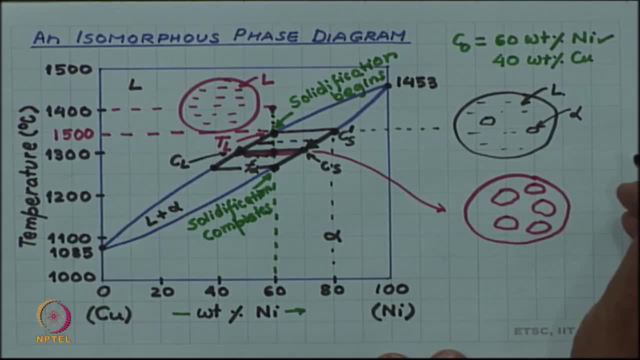 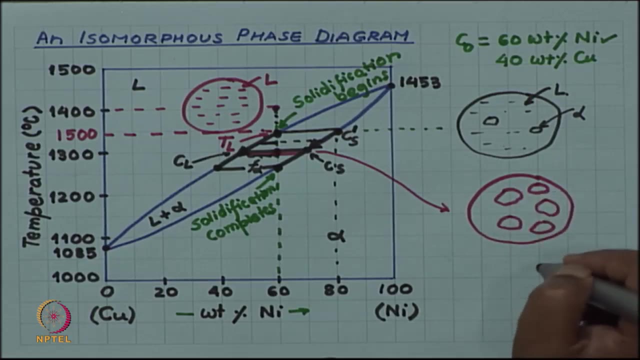 one point and that particular point will gradually grow into a single, continuous solid mass. So solid begins to form at different locations- This is called nucleation, and we will discuss that in detail later- and then those regions gradually develop. So you have several solid regions developing in the liquid phase. 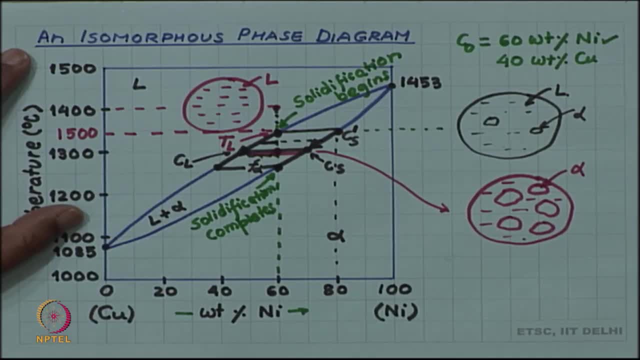 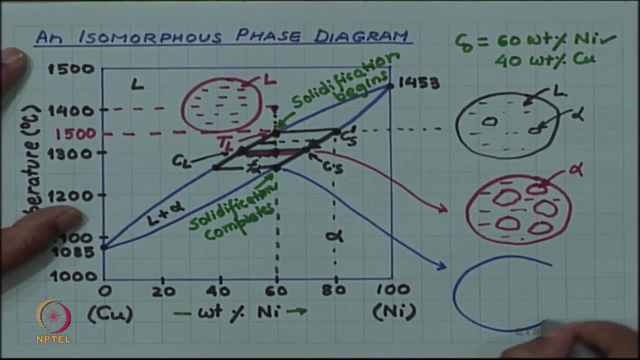 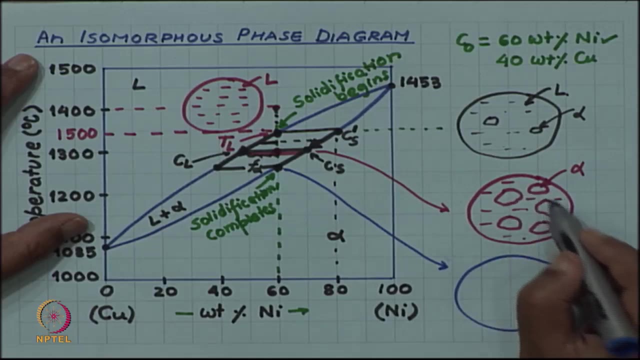 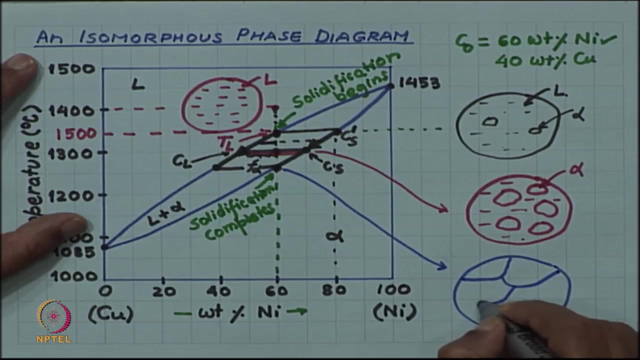 And finally, when you come to this, come to this last point: solidification has completed, So you have single solid phase. But then you can see that since the nucleation began at several locations, each of them will have their own region in the final microstructure. So 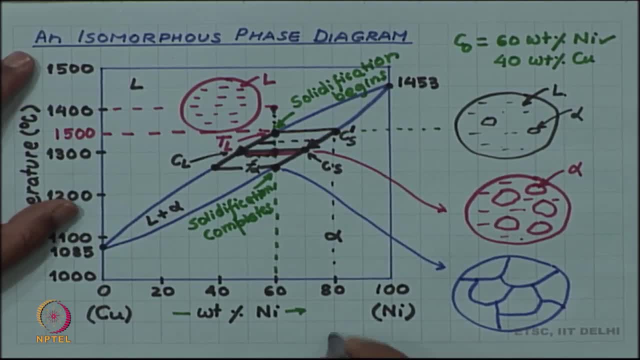 this is what we had earlier called, when discussing the surfaces and grain boundary, as a polycrystalline, polycrystalline polycrystalline system or a polycrystalline sample. So what you finally get is a single. 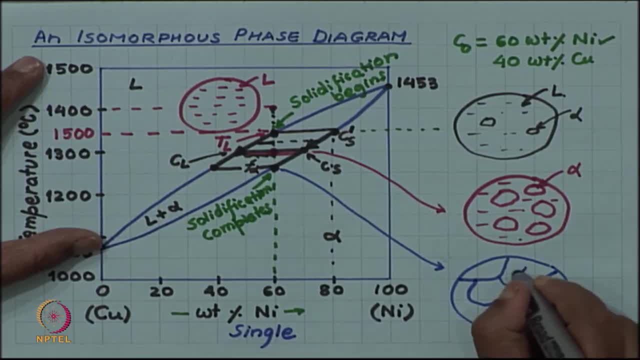 phase phase is same because each of them is alpha, all of them is alpha, but the difference is in their crystallographic orientation. So if I try to mark some sort of unit cell in them, because each is a crystalline phase- copper and nickel, if you remember, both are. 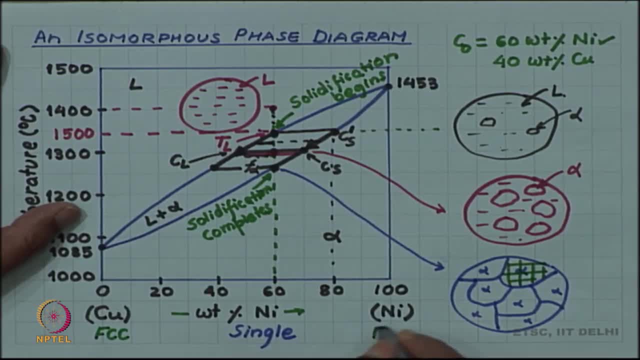 FCC. So these are the two components, And recall that we had talked about Hume-Rodry rule. So somehow copper and nickel satisfy the Hume-Rodry rule and that is why they are able to form a continuous, solid solution. Whenever you have an isomorphous system, you have a continuous.